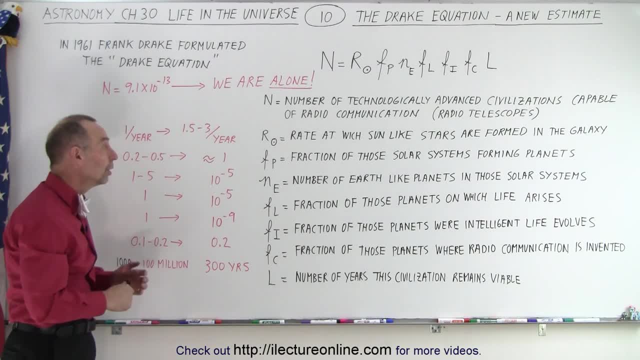 planets around it, At least one planet. So there we go. The fraction of those solar systems forming planets is probably much closer to one than it is to 0.2 to 0.5.. So so far, much more optimistic in this case. But now things begin to change. When Drake estimated that from 1 to 5 planets around 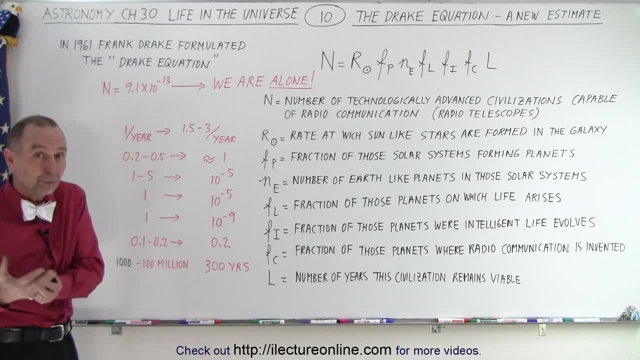 each star, that's that around each star that formed planets were earth-like planets. the estimate now went down to 10, to the minus 5. One in a hundred thousand, Because now we've already discovered thousands of planets and not a single one appears to be earth-like. There's 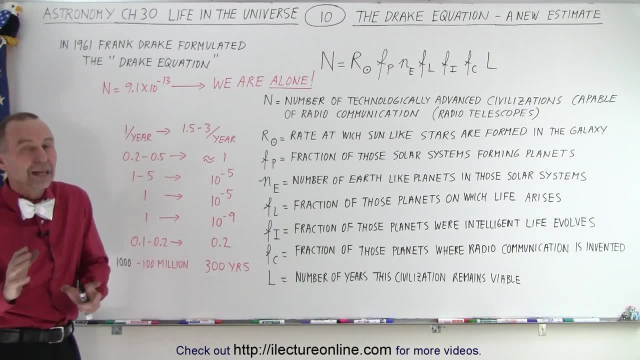 one, maybe two, that might be a little bit kind of like the earth, But truly like the earth the way it is, with oceans and air, the way we have it today. We haven't found one yet and the chance of one being found is much more remote now that we. 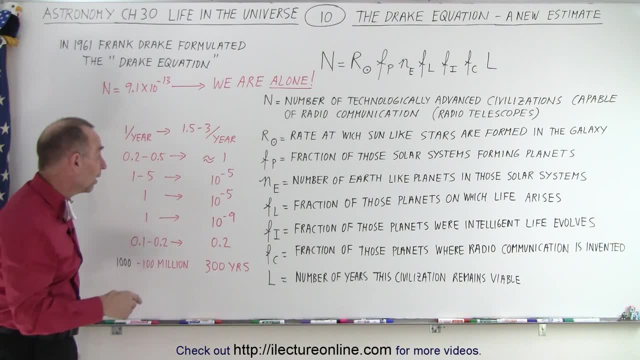 realize we have the technology to figure these things out, And so the probability has gone way down. And then of those planets, the fraction of those planets where life actually arises, we begin to realize how almost miraculous it is that there's life on the earth. We have no idea how it. 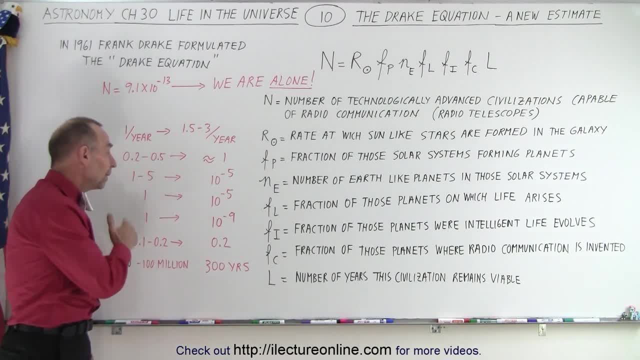 would be if life actually evolved on those planets, But it seems such an improbable event. So for those planets that are earth-like, the chance of life actually evolving on those planets is is also placed at a very, very, very tiny number Now of those planets where life evolves, and 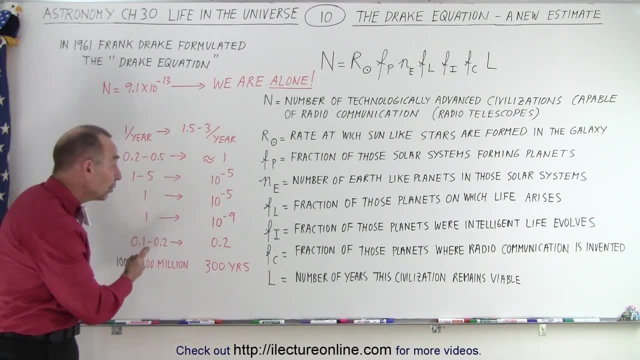 remember we had three billion years of essentially microbial life. that that would then turn into intelligent life, The chances are, again extremely remote. So the fraction of those planets that have intelligent life on it, the fraction of those that would then develop radio technology, well, that would be pretty high, because once there's, 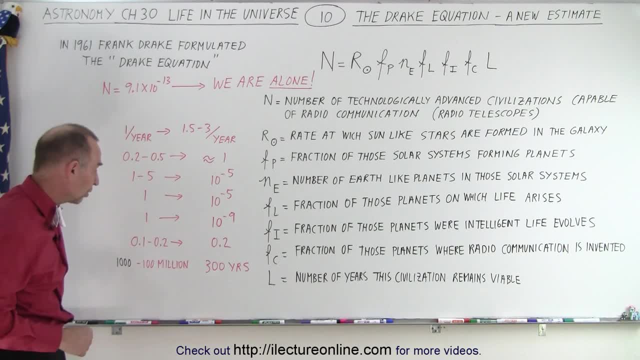 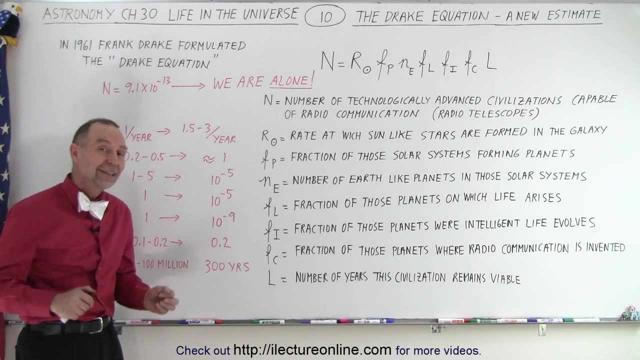 intelligent life, we think it would be fairly reasonable that they would develop the kind of technology they can communicate with. But then another very pessimistic result: Once a civilization is capable of producing radio technology, they're also capable of producing chemical weapons, biological weapons, nuclear weapons. They know what other weapons we're going. 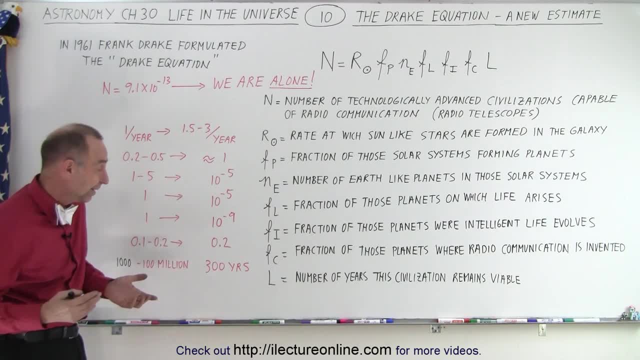 to be able to communicate with. We have all kinds of ways of destroying ourselves and our planet. The estimation is that there's only about 300 years to go before we will annihilate ourselves. Well, hopefully we'll break that particular estimate. We will not annihilate ourselves. 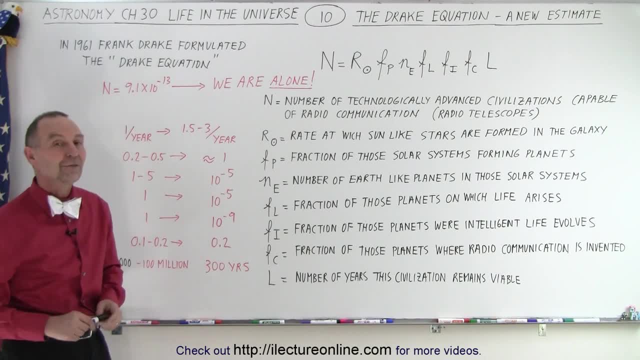 in the next 300 years. But again, when you take these very pessimistic views on the probability of a planet existing in our galaxy that we'll be able to communicate with, Well, it went down to 9.1 times 10, to the minus 13.. There's virtually no possibility of a planet being out there. 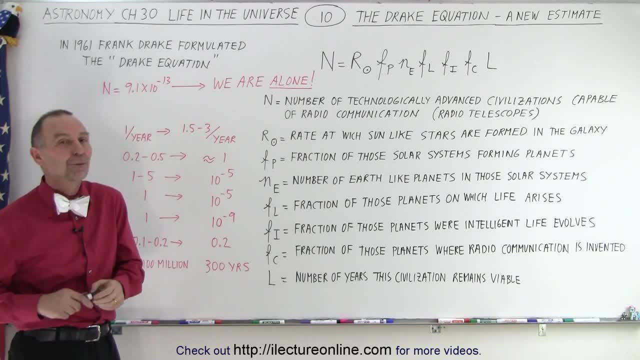 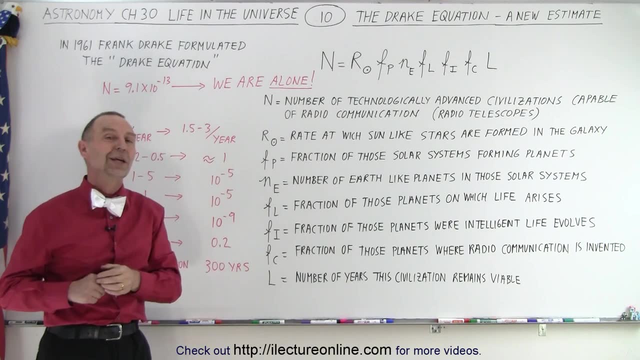 with intelligent beings capable of communicating with us, And if they're correct on these estimates, then we can say we're probably alone in our galaxy And there wouldn't be very many places in our universe where intelligent beings exist that could communicate with other intelligent beings. 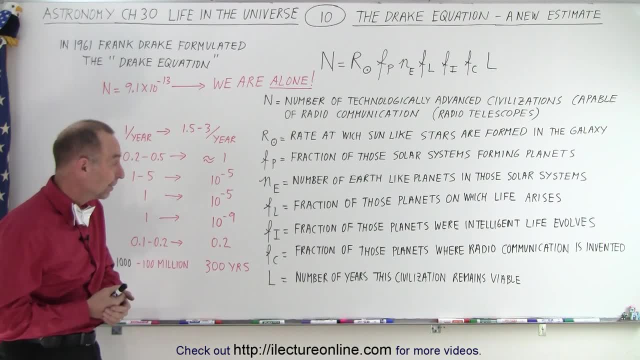 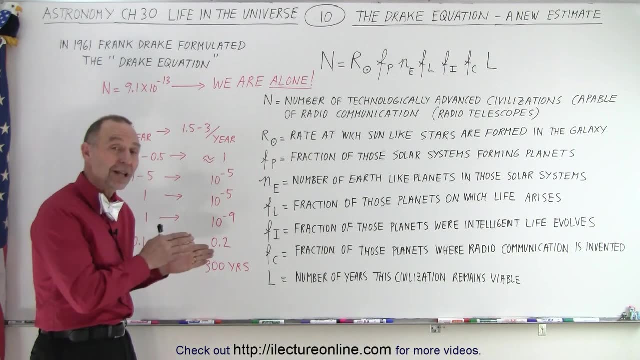 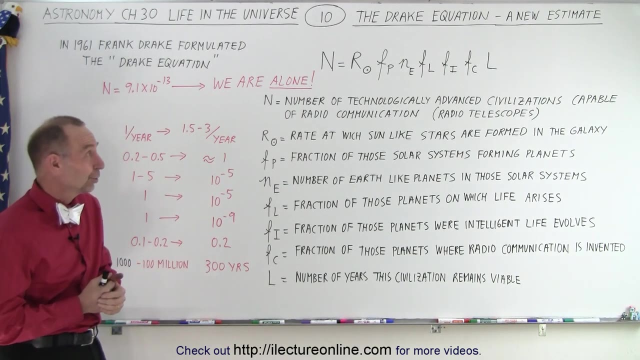 Hmm, that's a very different picture on the matter, But again, these are just theoretical estimates. It's probably somewhere between what Frank Drake taught in 1961 and these numbers right here, which are probably a little bit too pessimistic. Who knows? The key, I guess, is going to be: 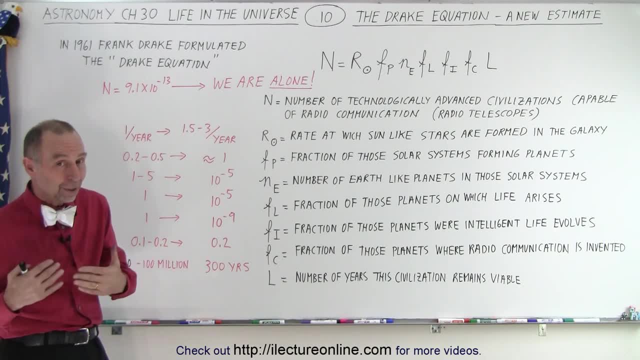 figuring out how life began on the earth. Once we can figure that one out, Once we can show how it how it happened- and it seems reasonable to believe that this can happen another planet- then we might have a much better estimate. But until we do it's still a big mystery. 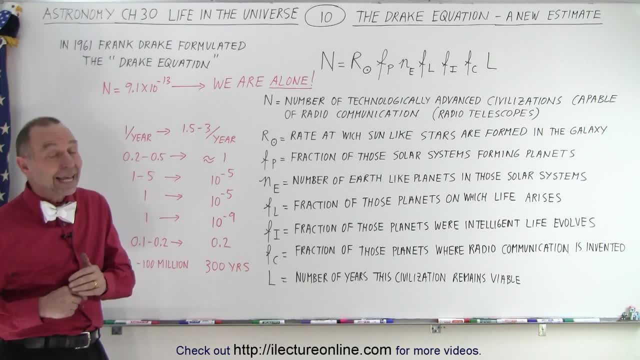 So how many years have we had the radio? Since the 1950s? So 1950s is when we began with radio communication. So we haven't had it for that long. We've had it for 70 years, Yep, 70 years. 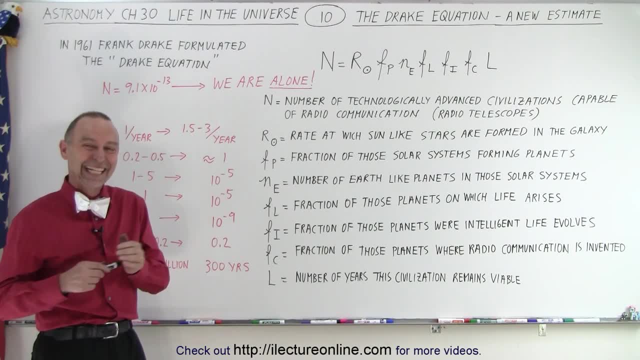 280 or 230.. 30 years left to go To restore ourselves. Yes, Imagine where we will be with our weapons technology in 230 years And who will have those weapons, and how will we relate to one another in this world? 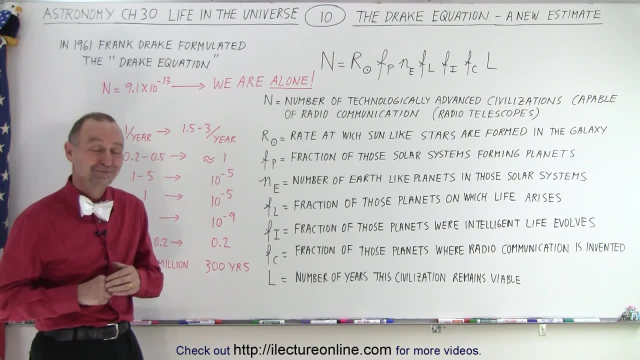 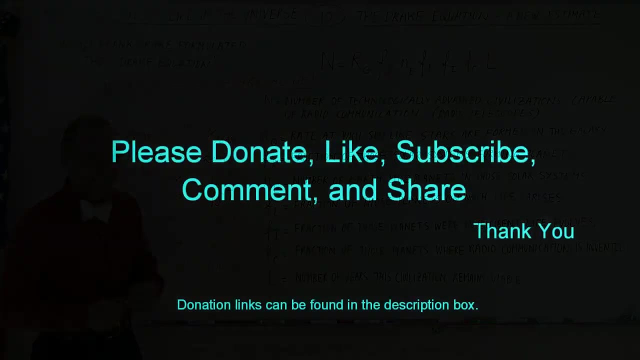 At this point in time, it's not looking good. Yeah, We still need to learn how to live with each other. unfortunately, We just can't get along. Yes, just look at us. You don't have to live with us, We'll make it up to you. 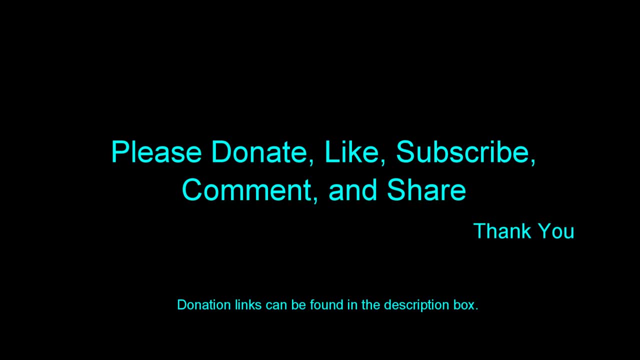 We'll try not to compare ourselves. My son will be so happy, Dad will be so happy. I can't even accommodate him now. I haven't even had to look at him in 30 years. This is what my son is like. I would have nothing to do with him if I didn't know he was crazy. I wouldn't have made a mistake in my life. I would have been the same if I had known I would have been as grown up. I've always wanted to try. I've had to be the best. I've always been the best. I've been there. I've been there.